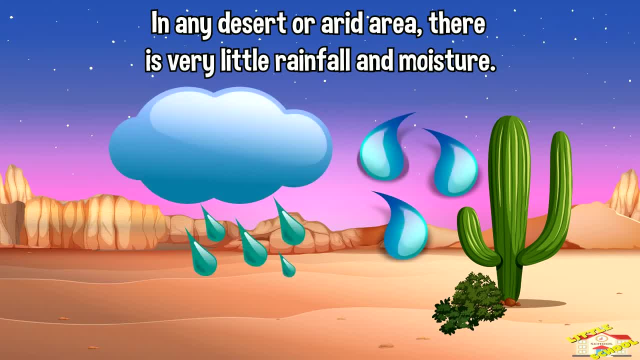 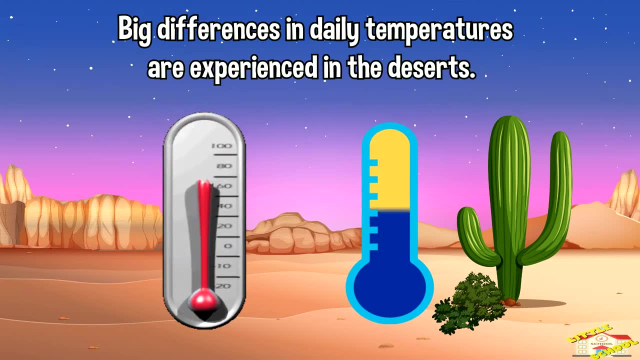 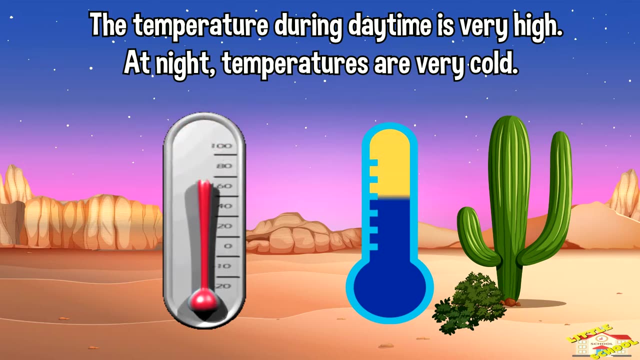 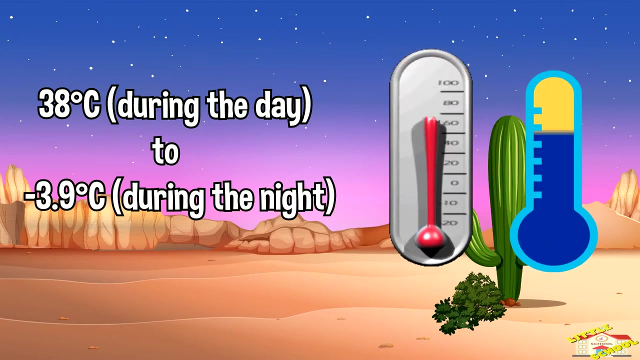 is very little rainfall and moisture. Big differences in daily temperatures are experienced in the deserts. The temperature during the sunshine hours are usually very high, while night temperatures are cold. Average temperatures range from 38 Celsius during the day to negative 3.9 Celsius during. 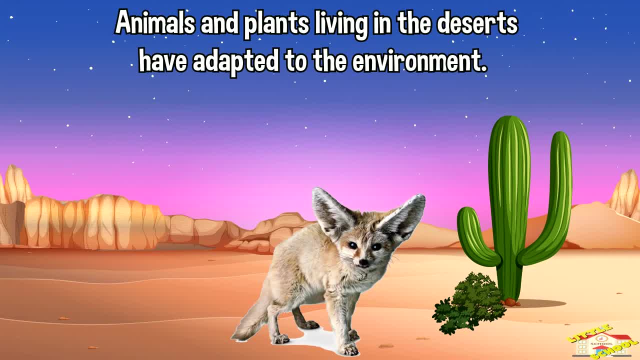 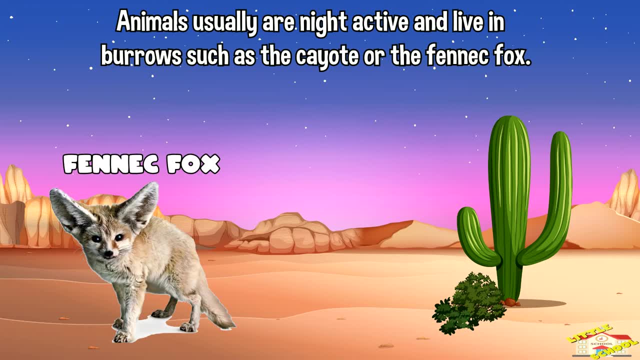 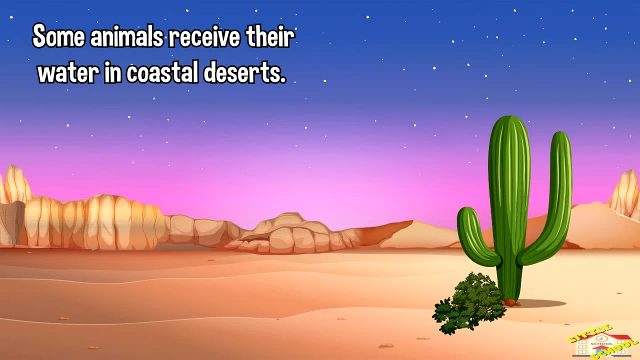 the night. Animals and plants living in the deserts have adapted to the environment. Animals usually are night active and live in burrows, such as the coyote or the fennec fox. Some animals receive their water intake from the water in coastal deserts or store. 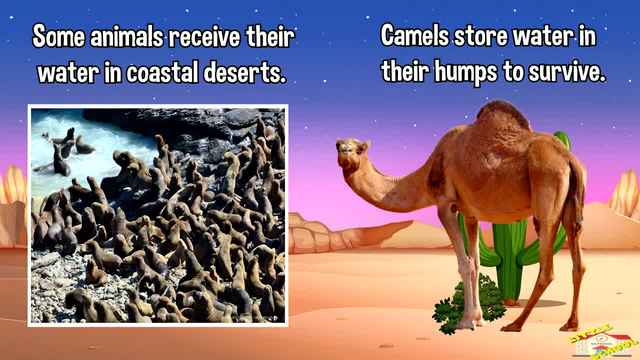 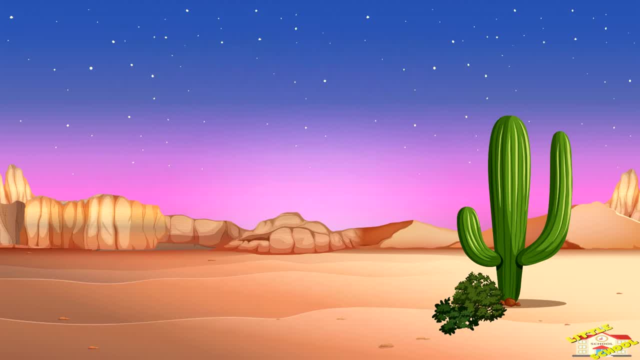 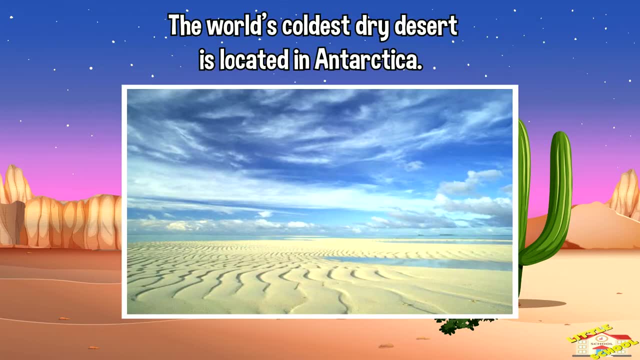 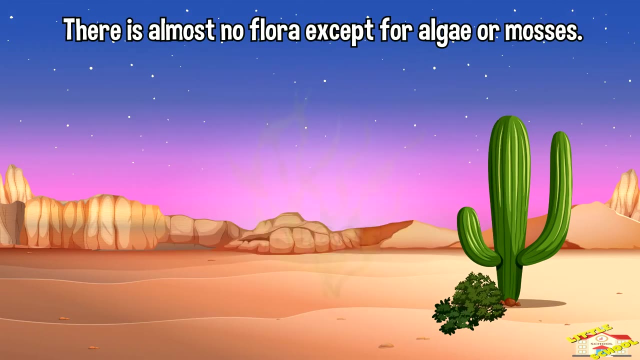 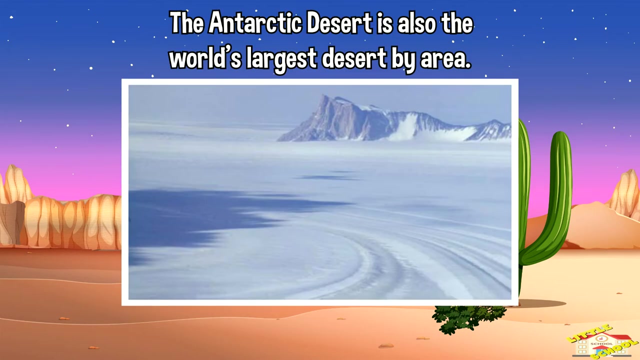 water in humps such as the camel. There are 12 deserts you should be familiar with. First is the Antarctic desert. The world's coldest dry desert is located in Antarctica. There is almost no flora except for algae or mosses. The Antarctic desert is a desert. 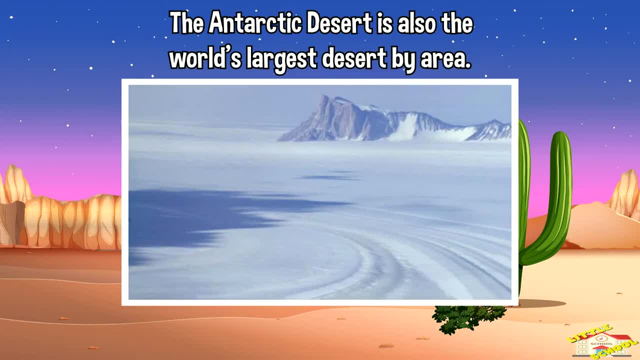 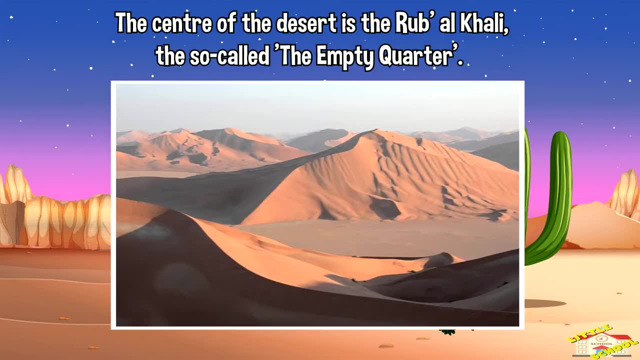 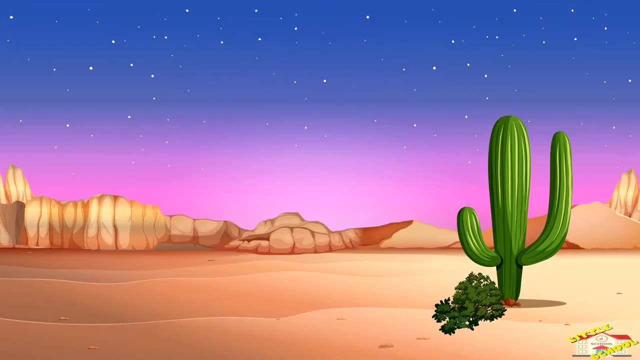 that is also the world's largest desert by area, The Arabian desert. The center of the desert is the Rube al-Khali, the so-called the Empty Quarter. The sand here has a red-orange color and the terrain is covered mainly by sand dunes. some 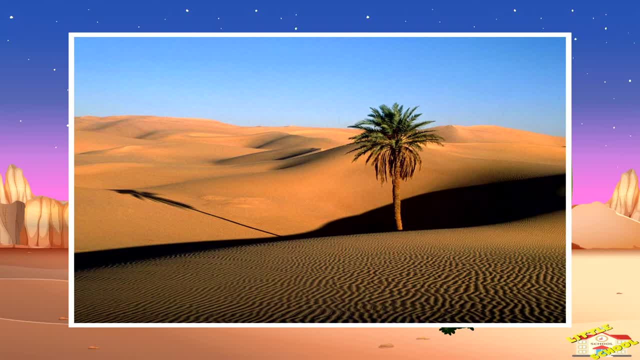 gravel plains and rocky plains. The Aralcum desert. The sand has an abundant amount of water content. The area is rich in hydrocarbons, zinc, zinc and zinc. It is the largest desert by area. The desert is also the world's largest desert by area. 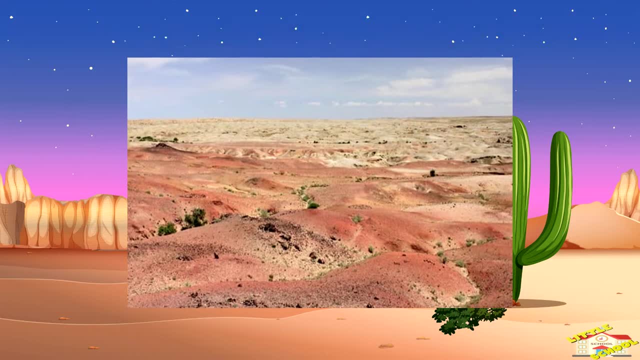 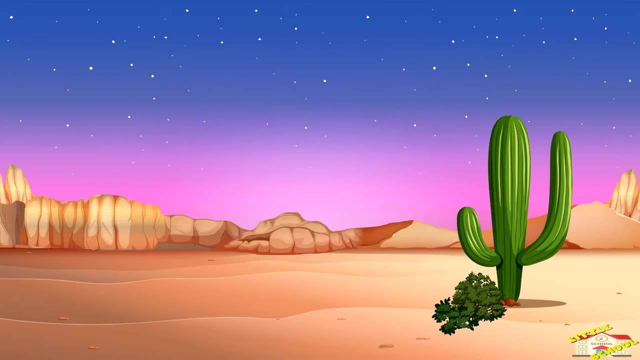 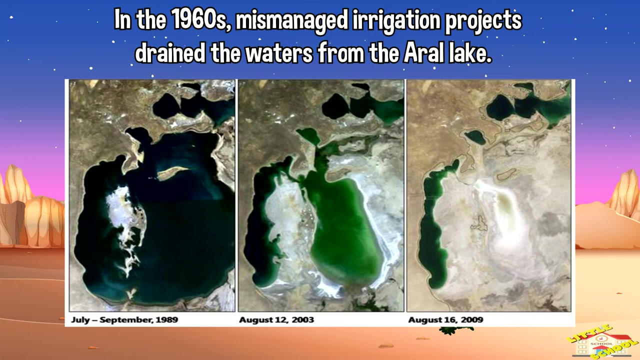 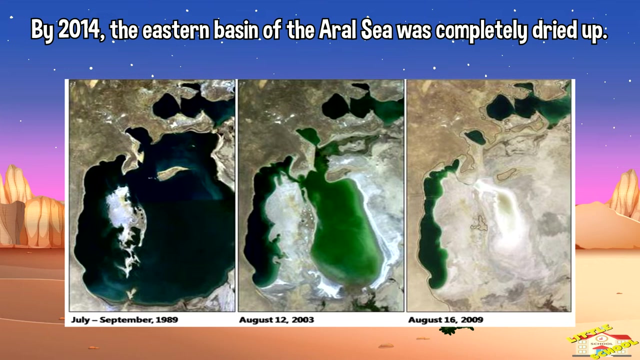 Aralcum Desert. The Aralcum Desert is known as the youngest desert of our planet. It formed in the 1960s, when irrigation projects for the huge cotton plantations in the area drained the waters from the Aral Lake. By 2014,, the eastern basin of the Aral Sea was completely dried up. 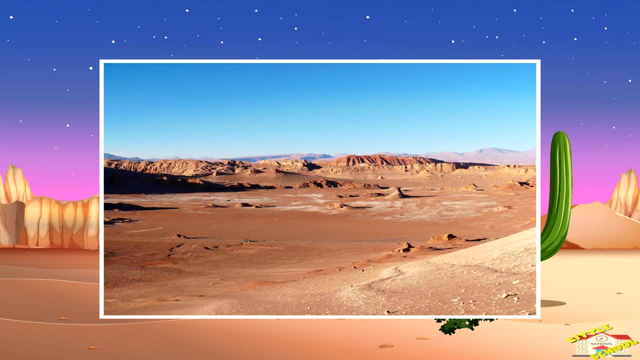 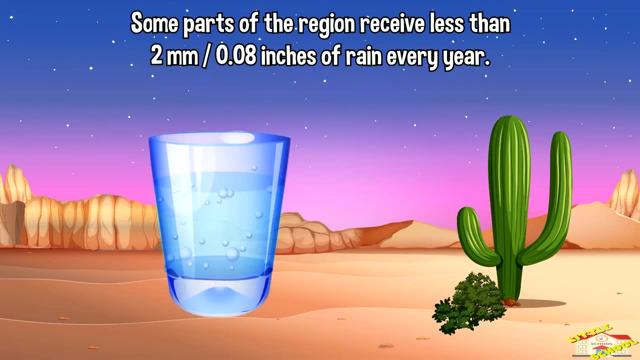 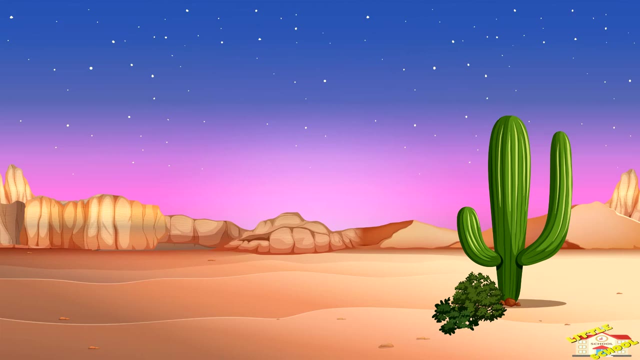 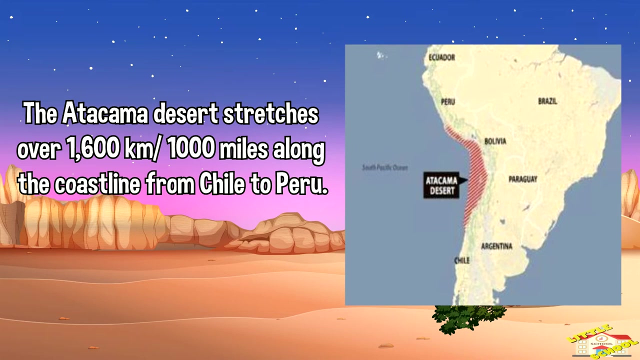 The Atacama Desert. This desert is known as the driest desert in the world. Some parts of the region receive less than 2 mm or 0.08 inches of rain every year. The Atacama Desert stretches over 1,600 km or 1,000 miles along the coastline from Chile. 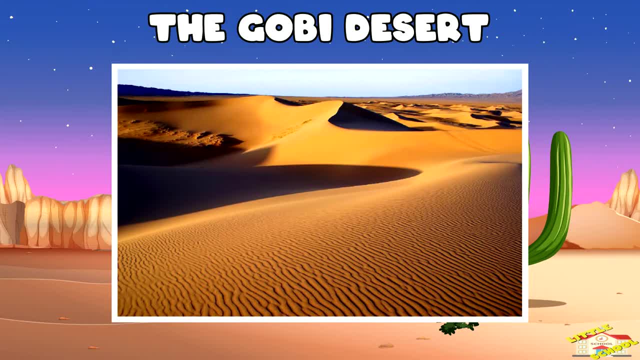 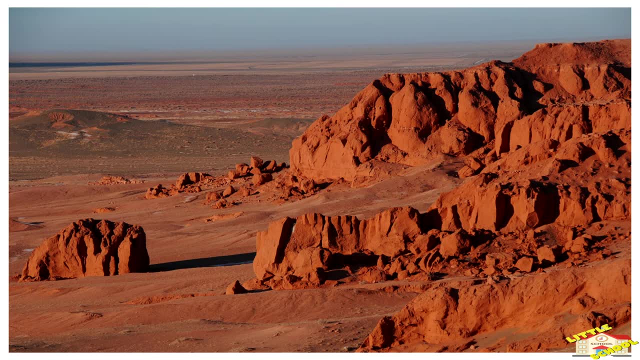 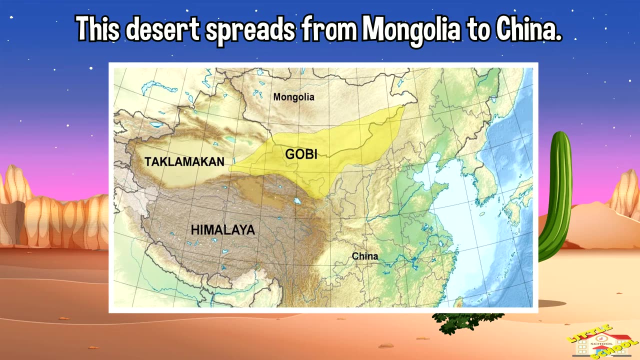 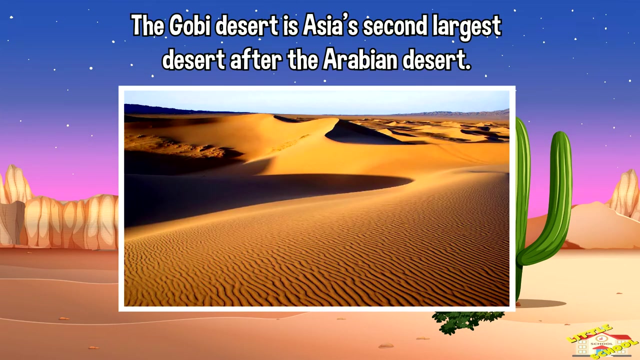 to Peru. The Gobi Desert. The Gobi Desert is located in eastern Asia and is the world's largest cold desert. This desert spreads from Mongolia to China. The Gobi Desert is Asia's second largest desert, after the Arabian Desert, The Mojave Desert. 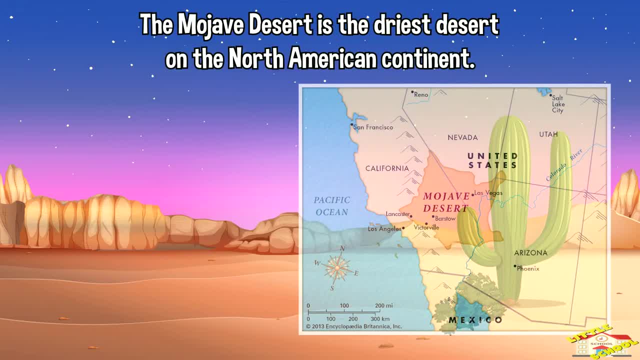 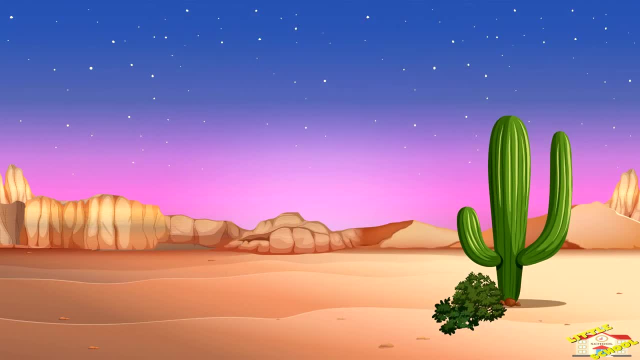 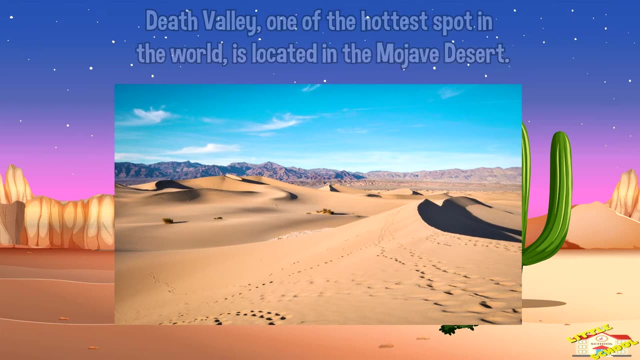 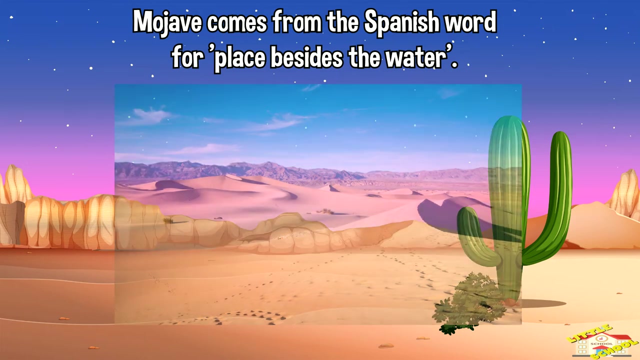 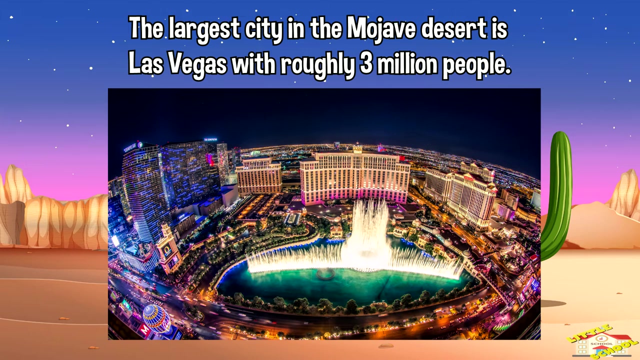 The Mojave Desert is the driest desert on the North American continent. Death Valley, one of the hottest spots in the world, is located in the Mojave Desert. Mojave comes from the Spanish word for place besides the water. The largest city in the Mojave Desert is Las Vegas, with roughly 3 million people. 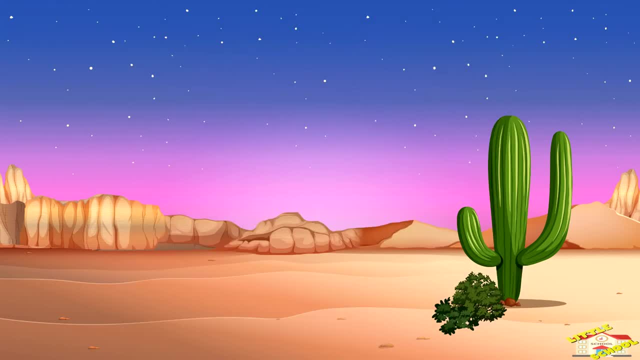 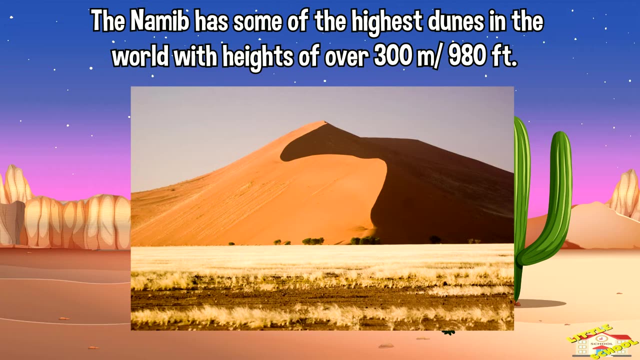 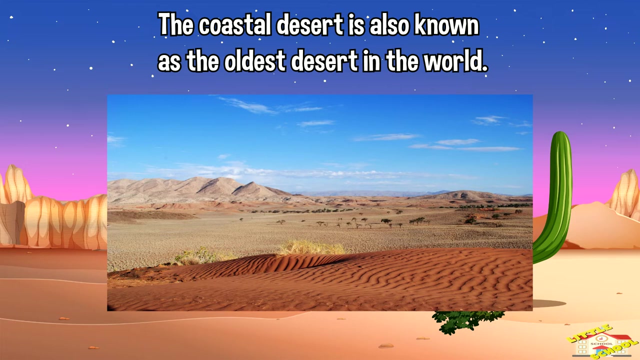 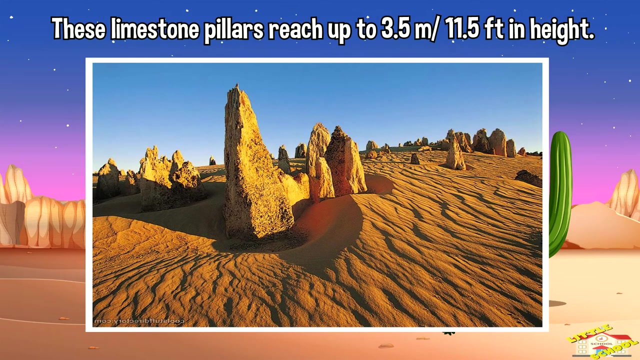 The Namib Desert. The Namib has some of the highest dunes in the world, with heights of over 300 meters or 980 feet. The coastal desert is also known as the oldest desert in the world: The Pinnacles Desert. The Pinnacles in Nambung National Park are limestone pillars and some reach up to 3.5. 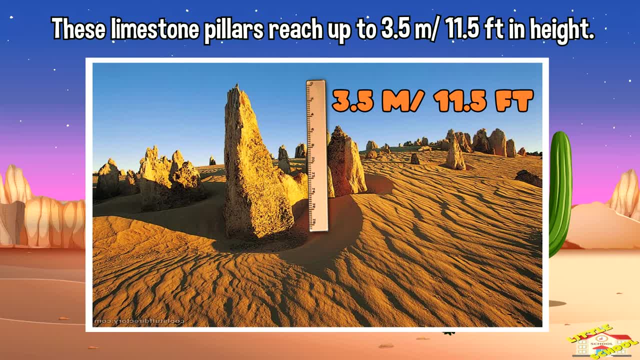 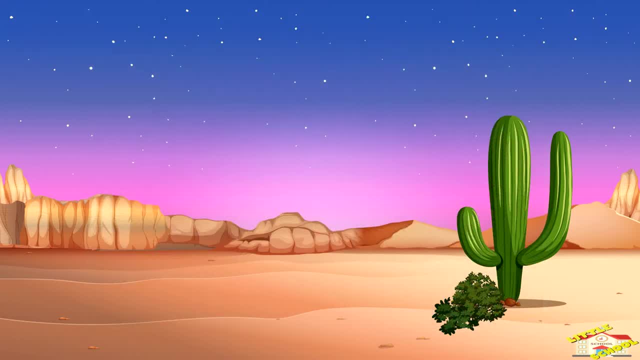 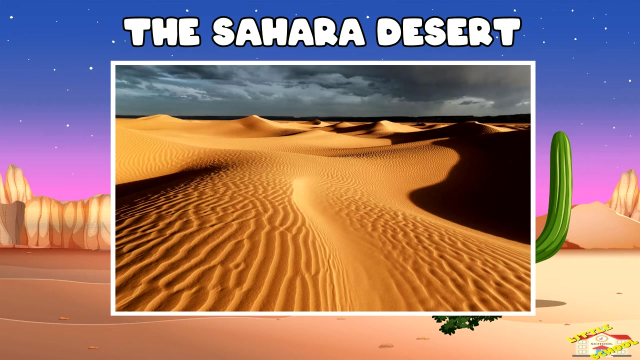 m, or 11.5 ft in height point. five feet in height, Wild emus can be found in this desert. This desert is only a small Australian desert, but it's known for its scenic landscape. The largest desert on Australia, however, is the Great Victoria Desert, The Sahara. 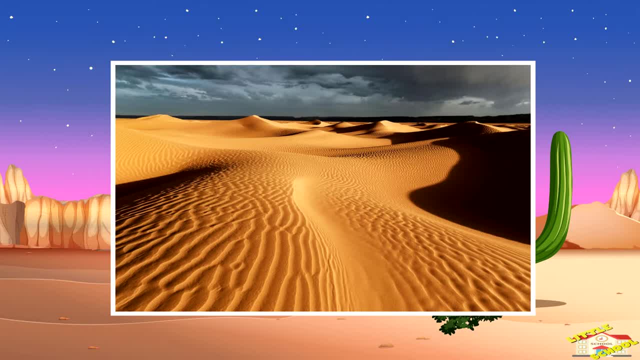 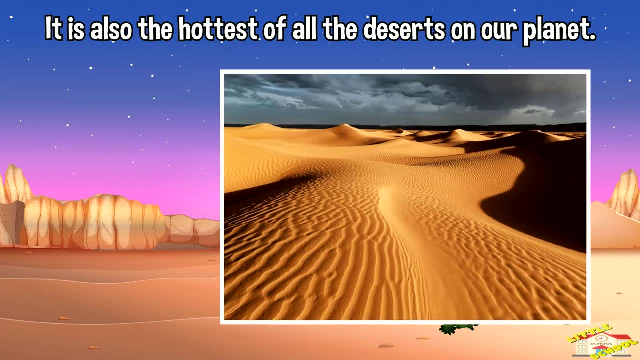 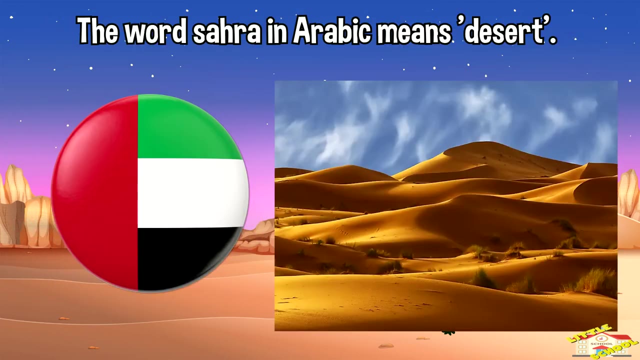 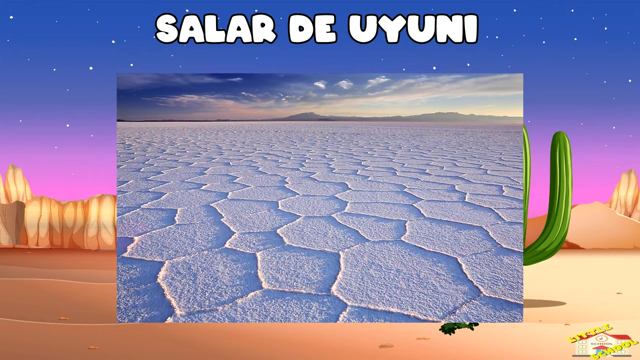 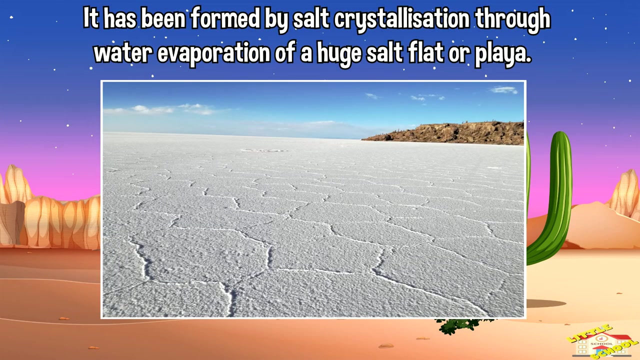 Desert. The Sahara Desert is the world's largest hot desert. It is also the hottest of all the deserts on our planet. The word Sara in Arabic means desert Salar de Ayuni. The Salar de Ayuni is a desert in South America that has been formed by 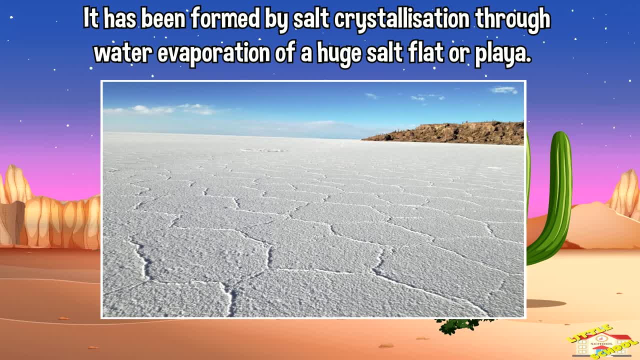 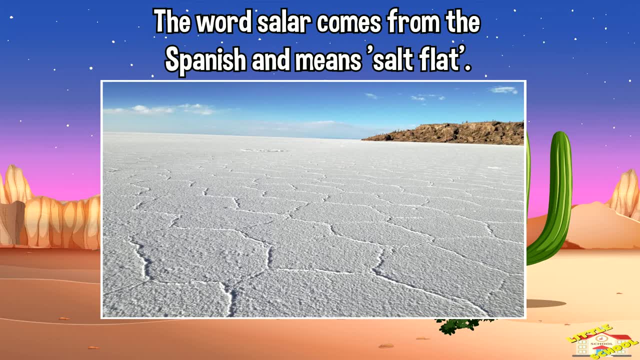 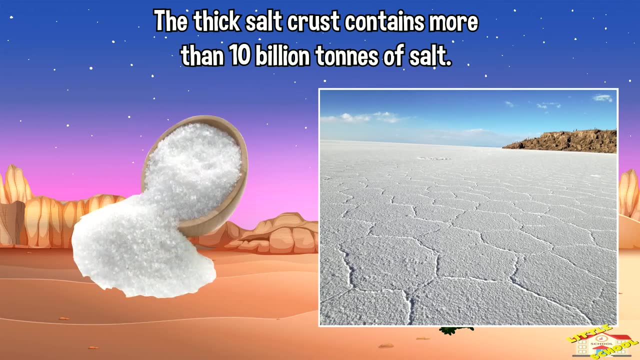 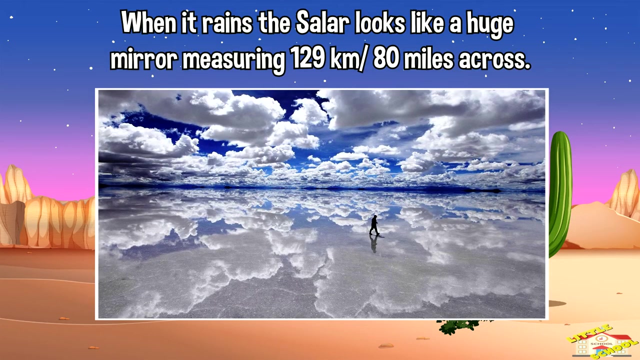 salt crystallization through water, evaporation of a huge salt flat or playa. The word salar comes from the Spanish and means salt flat. The thick salt crust contains more than 10 billion tons of salt. When it rains, the salar looks like a huge mirror. 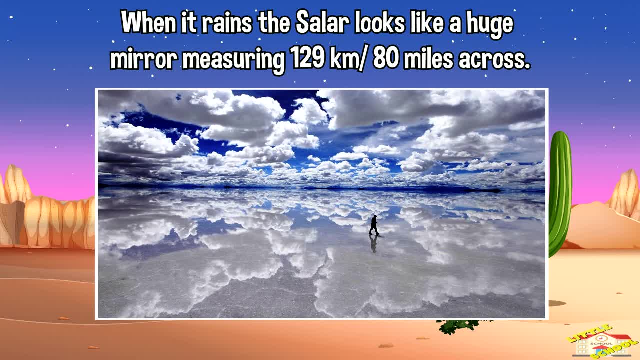 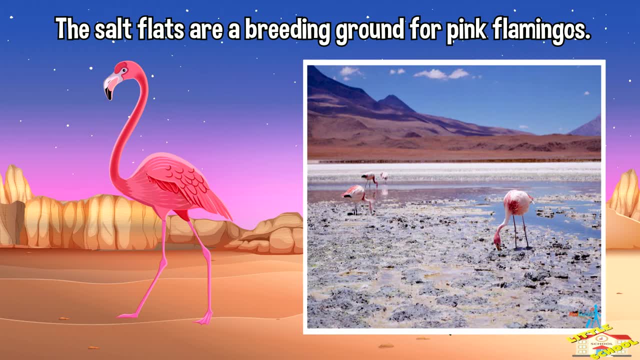 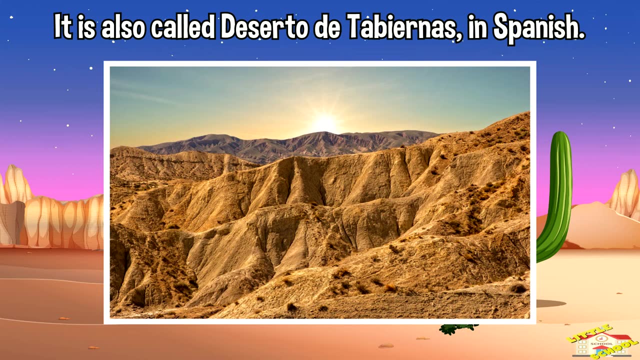 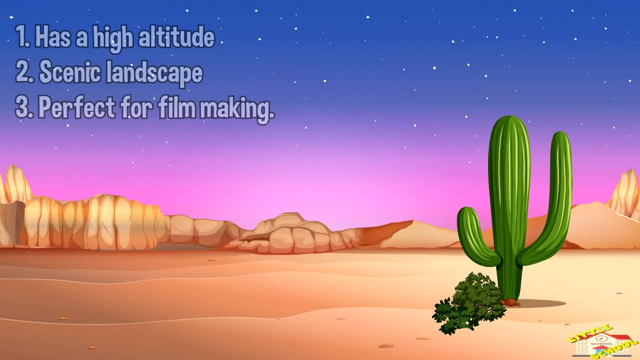 measuring 129 kilometers, or 80 miles across. The salt flats are a breeding ground for pink flamingos. Next is the Tabernas desert. It is also called Deserto de Tabernas in Spanish. The high altitude of the region and the scenic 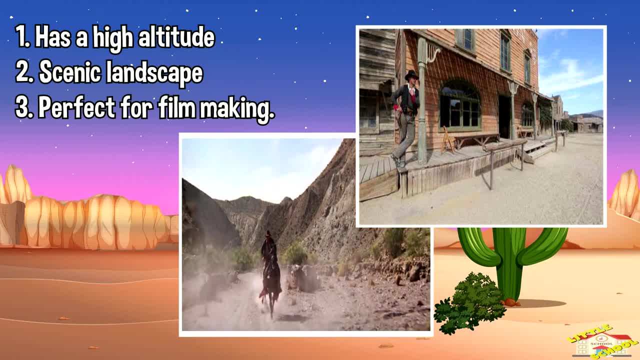 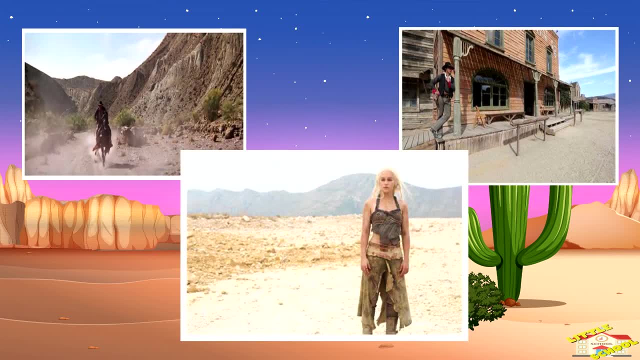 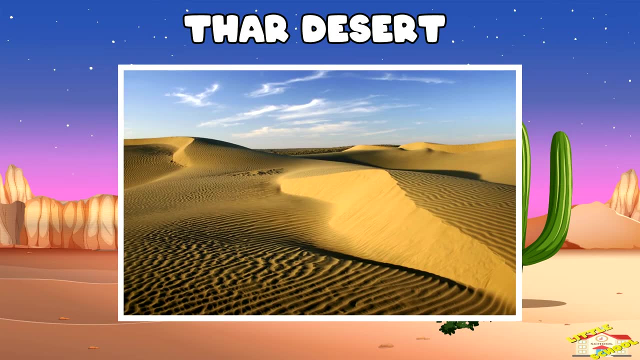 landscape of this desert has been beneficial for filmmaking. Many western-style movies, as well as one scene in the Game of Thrones series, have been filmed in a Tabernas. And finally, the Thar Desert. The Thar desert is known as the world's most densely populated. 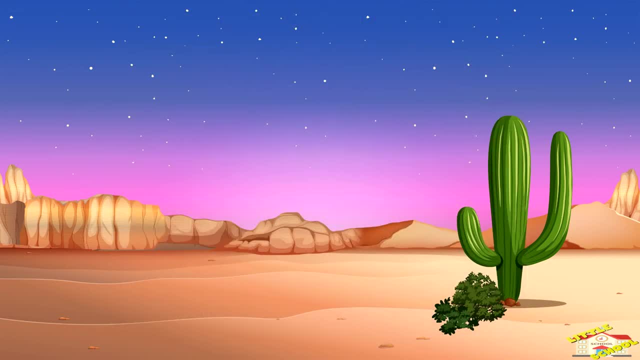 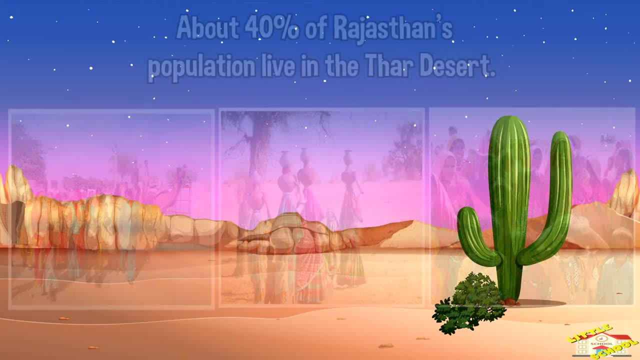 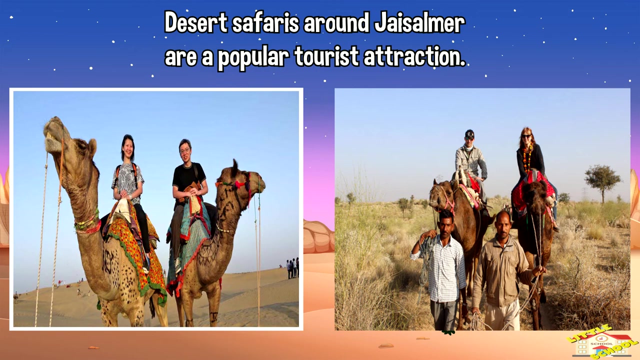 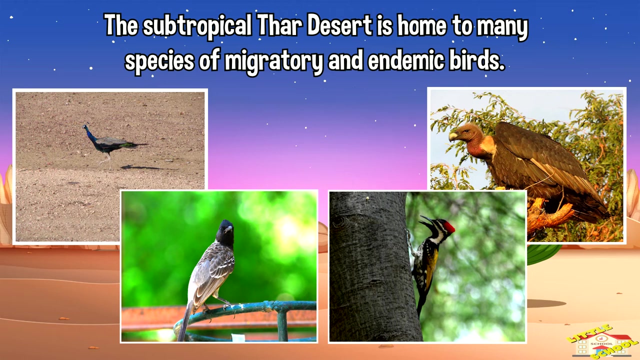 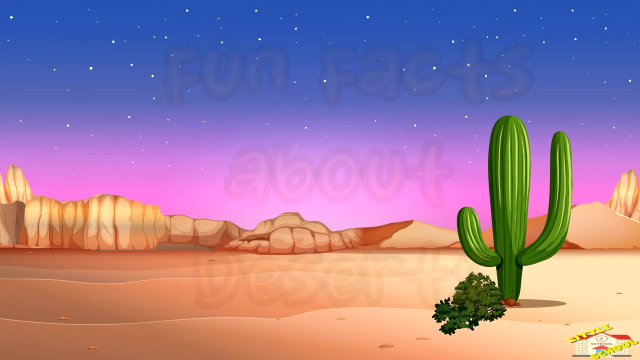 desert area. About 40 percent of Rajasthan's population live in the Thar Desert. Desert safaris around Jaisalmer are a popular tourist attraction. Subtropical Thar Desert is home to many species of migratory and endemic birds. Now here are fun facts about deserts. The five largest deserts in the world are: